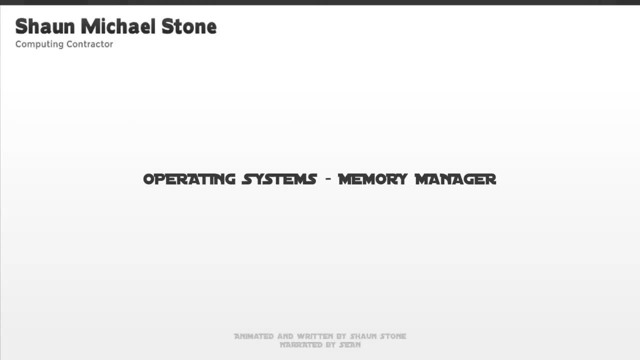 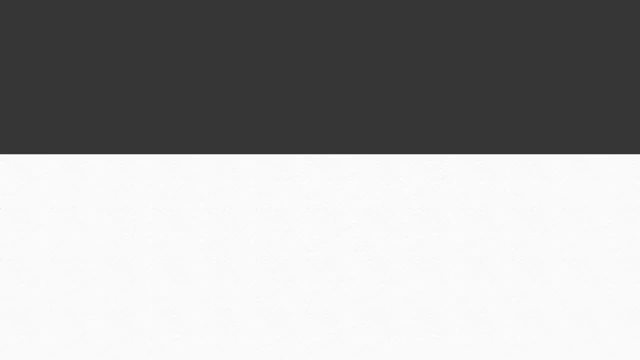 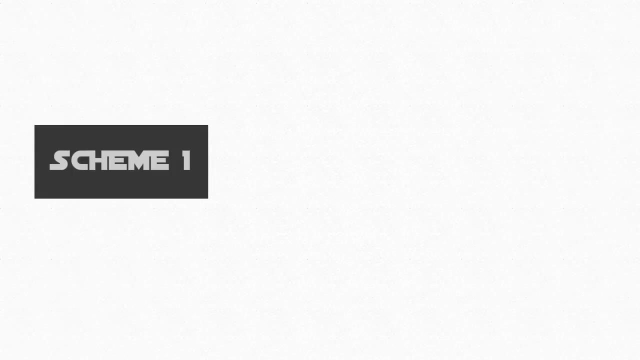 Hello, my name is Sean and in this tutorial we shall begin with the memory manager and look at three old schemes of memory management. Single user contiguous was the first scheme of memory management and it wasn't very efficient in terms of performance. A single 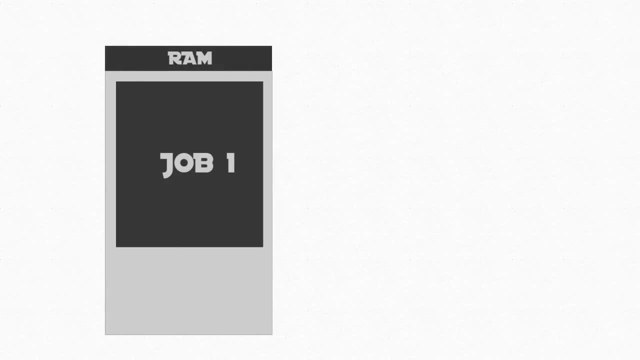 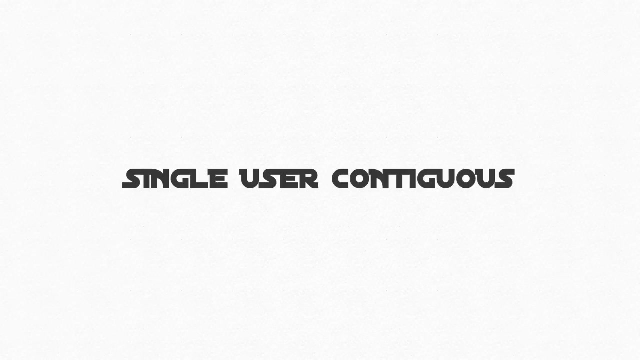 job would reserve the entire memory space. This job would be processed and then the memory was cleared, allowing the next job to be loaded. If the job size was larger than the space available in the RAM, it could simply not be executed. This scheme is considered. 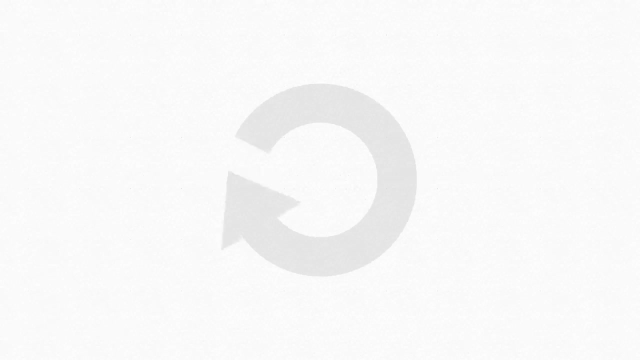 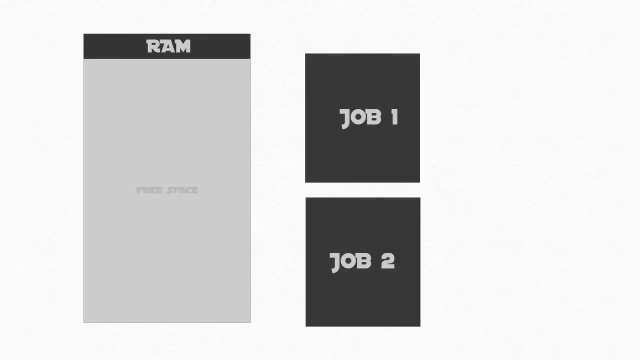 impractical for today's modern operating systems, as it would be very slow to process all of the jobs on demand. But what if you wanted to store two or three jobs in the memory? This is when fixed partitions came along, allowing allocated partitions to contain. 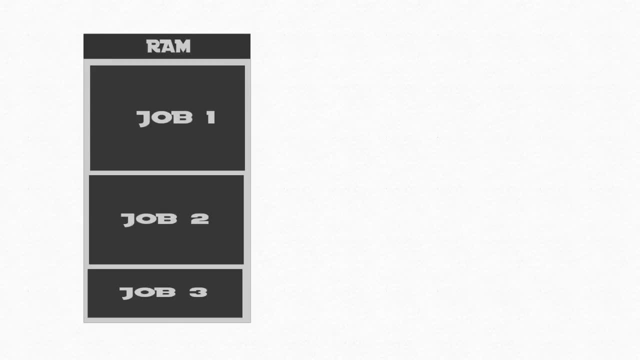 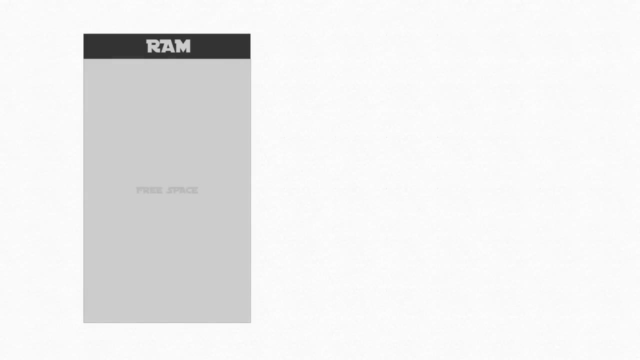 more than a single job at one time. All of the partitions were stored in a partition memory table to keep track of partition usage. The sizes of these partitions were static, meaning they could not be changed unless the system was rebooted. So you could see how this would be a problem. 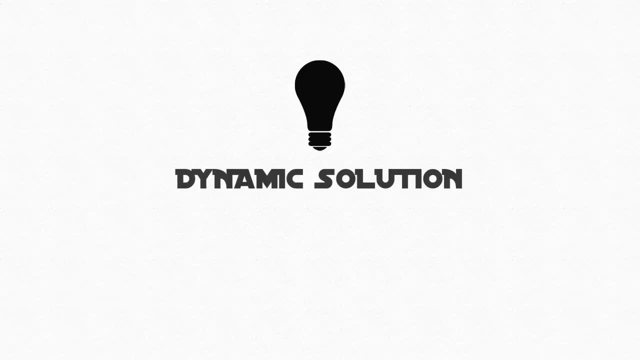 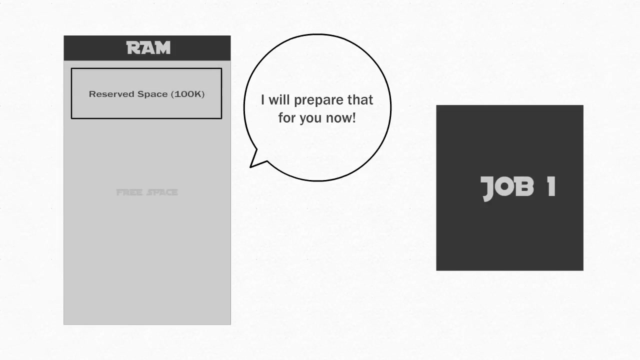 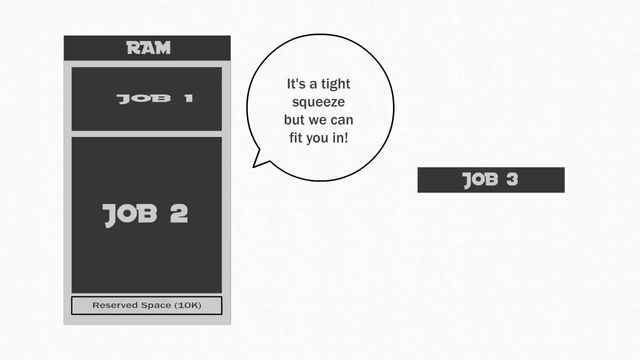 A dynamic solution was necessary to avoid having to reboot the computer every time you wanted to process a job. A dynamic partition's available memory is still kept in contiguous blocks, but jobs are only given as much memory as they request when they are loading for the processing. This has proven a significant improvement over fixed partitions, because 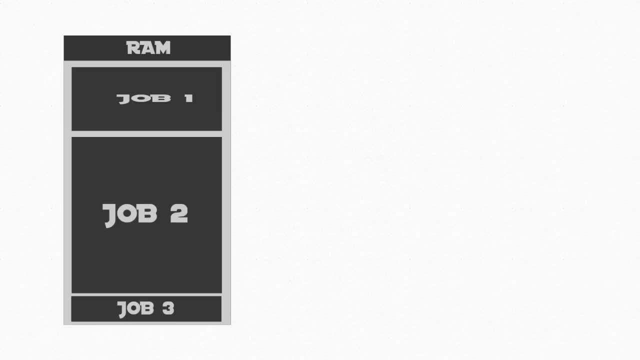 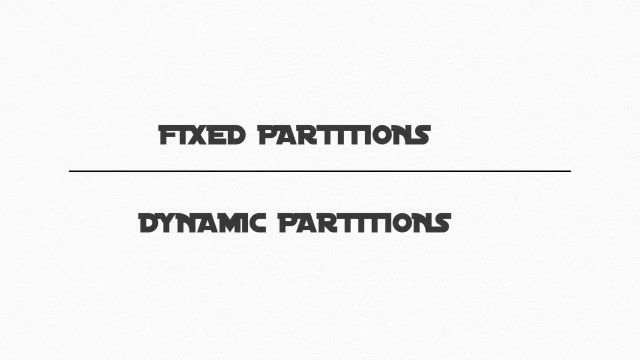 memory is not limited to just fixed partitions. This is a significant improvement over fixed partitions. The partition's memory is not wasted in the partition. Unfortunately, this is not a complete solution. Both fixed and dynamic partitions need some way to allocate jobs to the available. 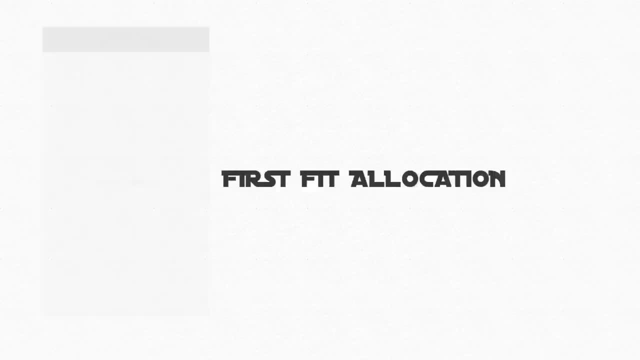 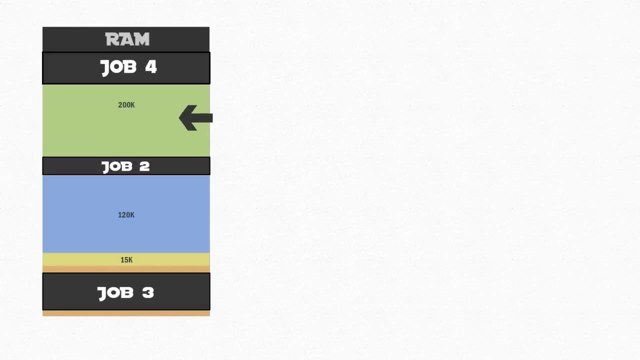 partitions. There are two ways to do this. The first fit quite simply finds the first partition that has sufficient storage space, not taking into account how much memory could be wasted in the allocated partition. The best fit first looks for the smallest partition, resulting in more space for other jobs, resulting in slower performance but better efficiency. 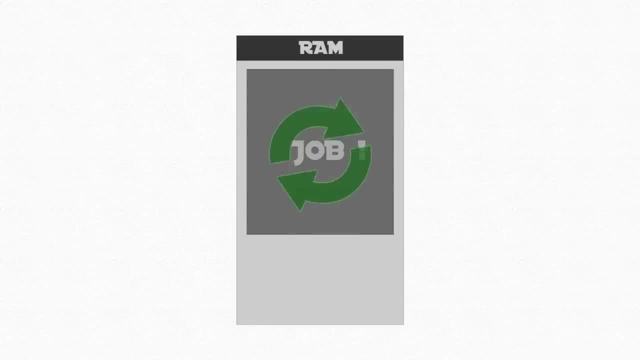 So when a job has completed processing, it is then removed from memory, also known as deallocation With a fixed partition. this is fine. it is simply cleared. But when using a dynamic partition it gets more complex to free up memory as it tries to join together. 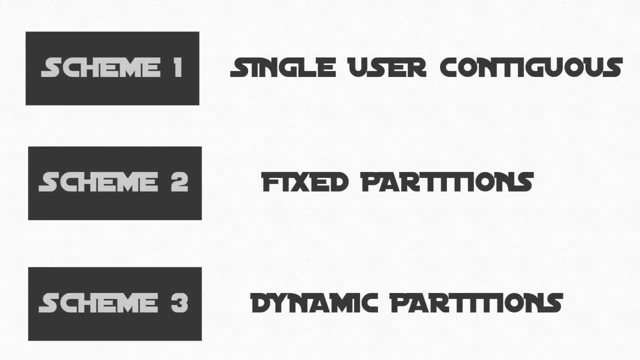 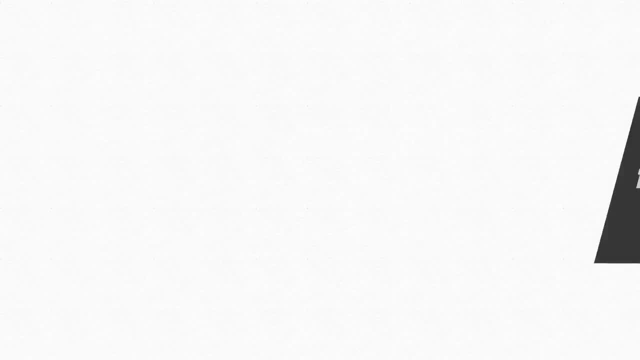 adjacent blocks. So looking at these six different partition options, we can see that the first one is the easiest. Looking at these simple allocation schemes, we can see there are still problems. Each one required the memory manager to store the entire program in the main memory at contiguous. 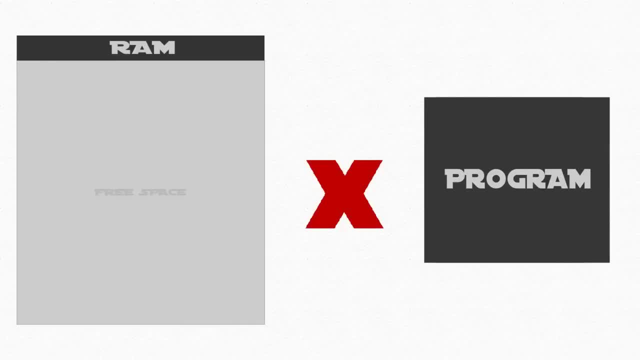 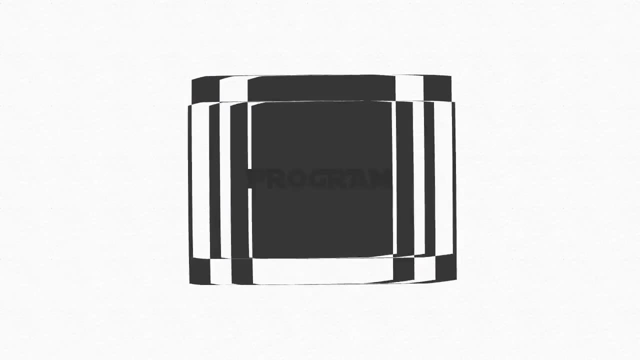 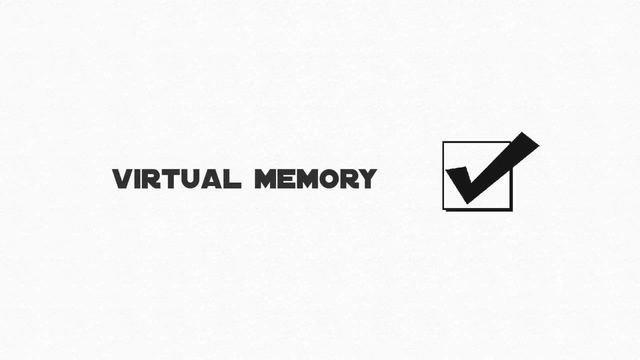 locations. We need to find a way to avoid having to keep the whole program in memory to run and the restriction of storing the programs contiguously. What if we could divide the jobs into separate, smaller chunks? We can. Simple memory is the solution and we shall look at the evolution of four memory allocation. 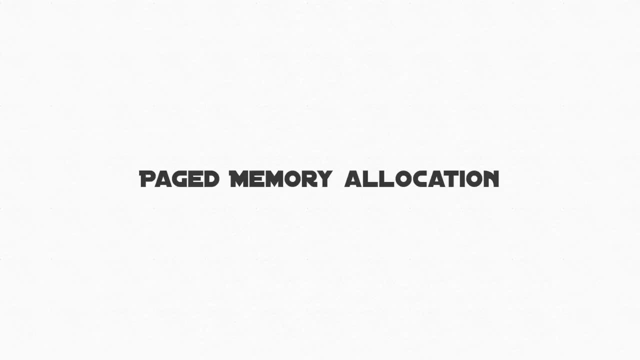 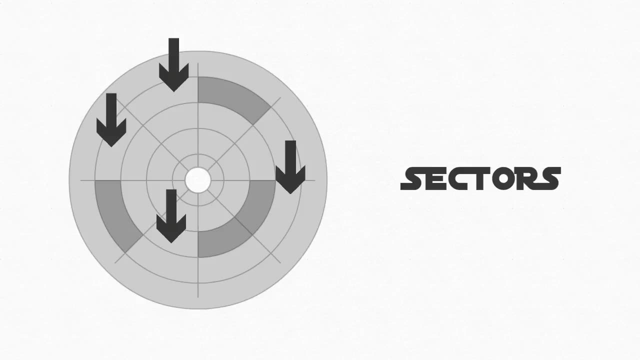 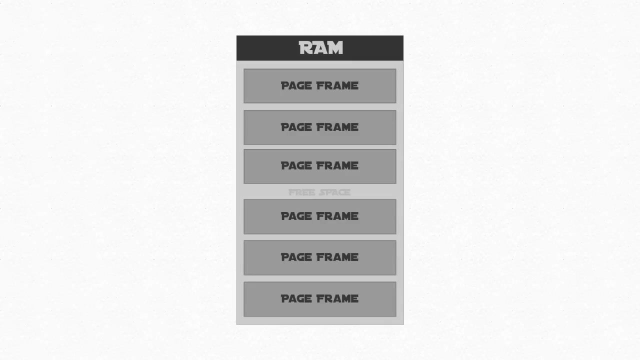 schemes. Let us start with paged memory allocation, allowing us to divide the job into equal-sized parts. The sections of a disk are known as sectors or blocks, and the sections of main memory are known as page frames. Before executing a program, the memory manager makes some preparations. 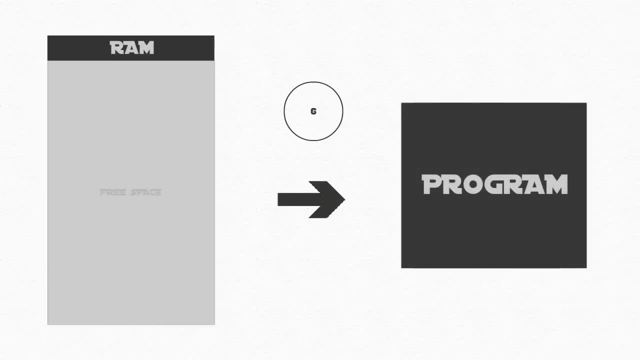 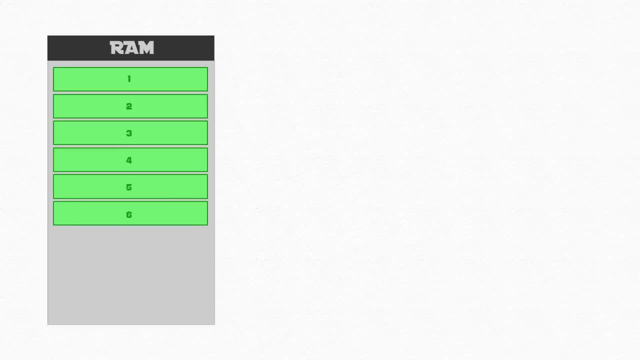 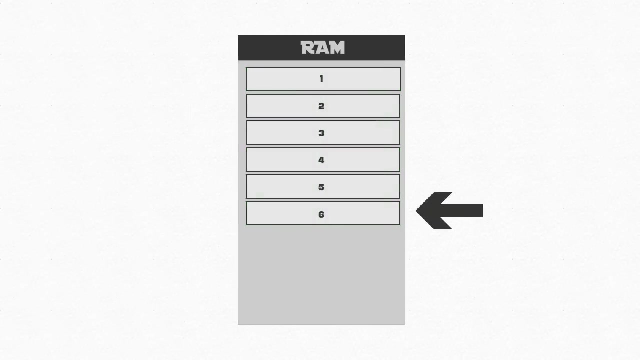 First it determines how many pages are in the program and then it locates enough empty page frames in the main memory so that it can pass all the pages into them. The adjacent memory blocks do not have to be loaded in as adjacent memory blocks They 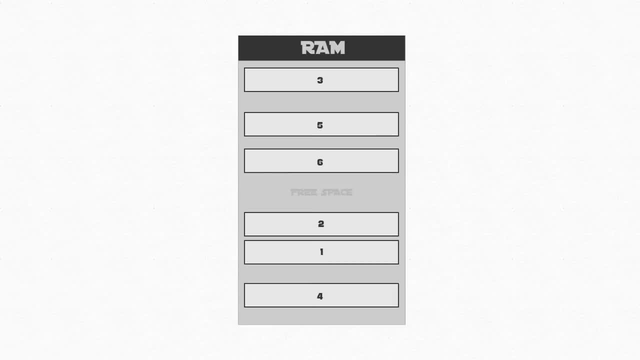 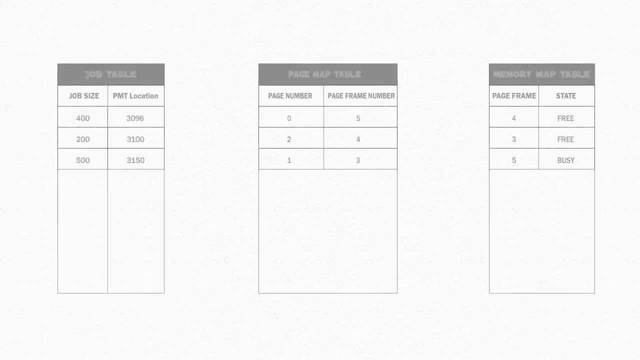 can be stored in any available page frame in the main memory. Now, this is a more efficient scheme, but it does come with complications. We need a way to keep track of all the page locations, which increases complexity in the operation, Through the use of three tables. 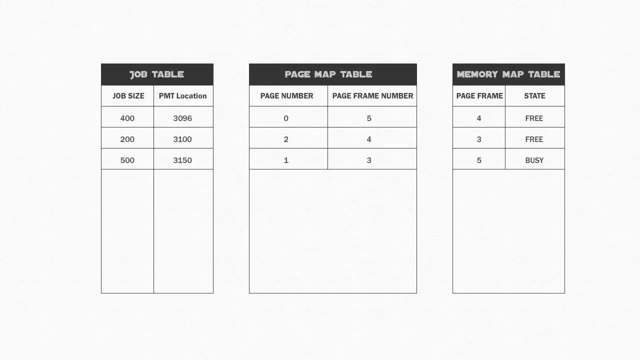 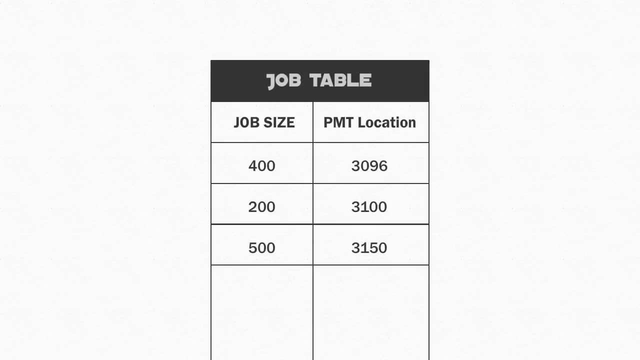 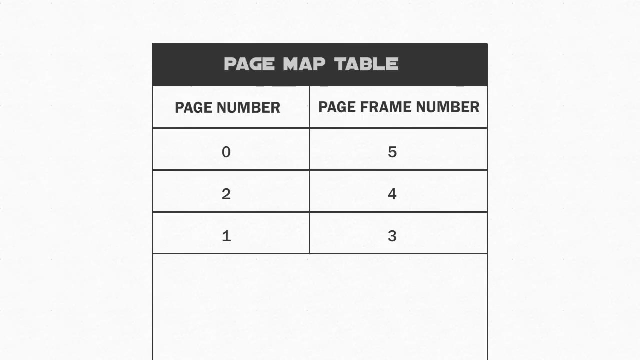 stored in the part of the main memory, we can keep an eye on locations of various jobs. The job table is a dynamic list that contains two values: the size of the job and the page map table location of that job. The page map table contains important information for each of the pages: the page number. 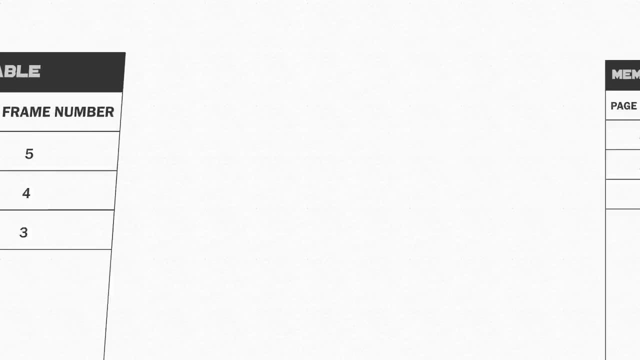 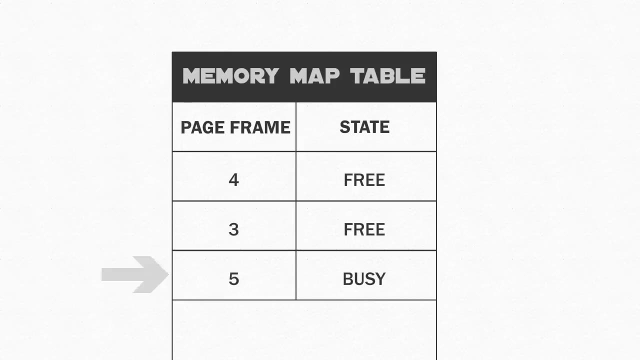 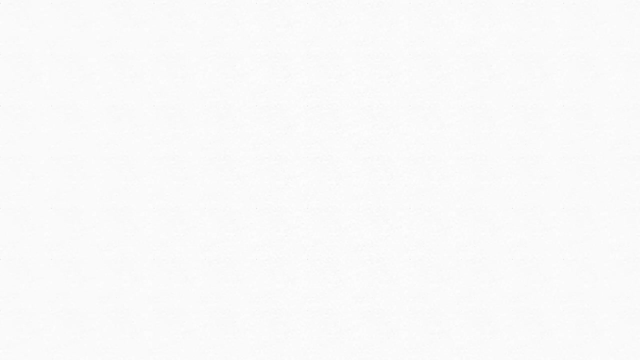 and its corresponding page frame memory address. Finally, the memory map table has one entry for each page frame listing both its location and a status informing whether it is in a busy or free state. Now that we have an understanding of paged map allocation, we can now see how demand paging. 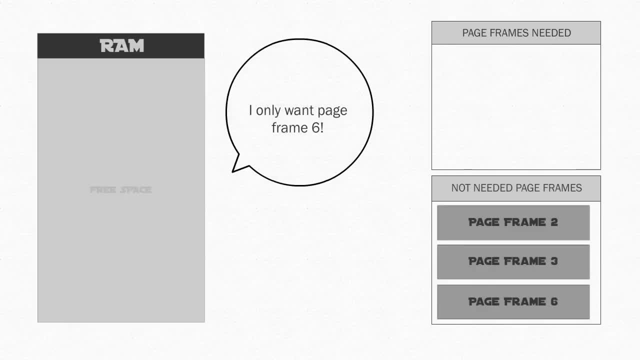 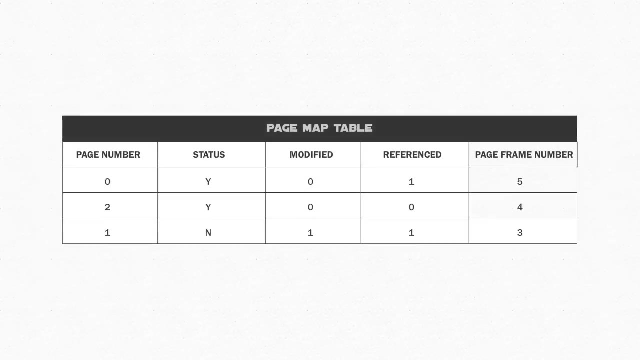 works. It's very similar to the previous concept, but the main difference is that pages are loaded on demand, Meaning that pages are only brought into memory when they are actually needed. The page map table we looked at before increases with three more columns: One to determine if the page is already. 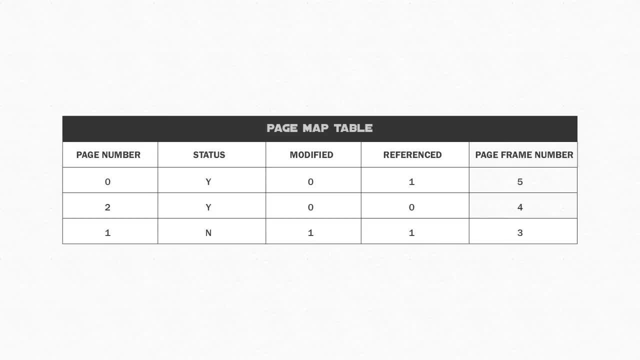 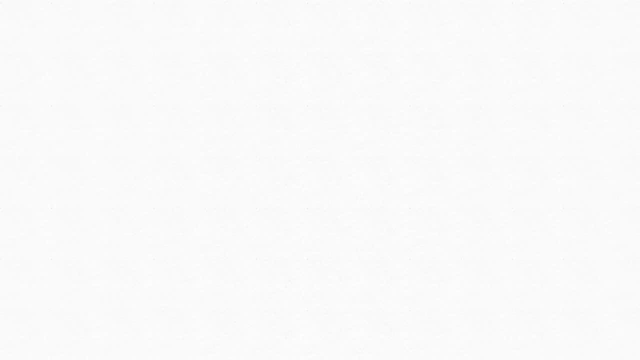 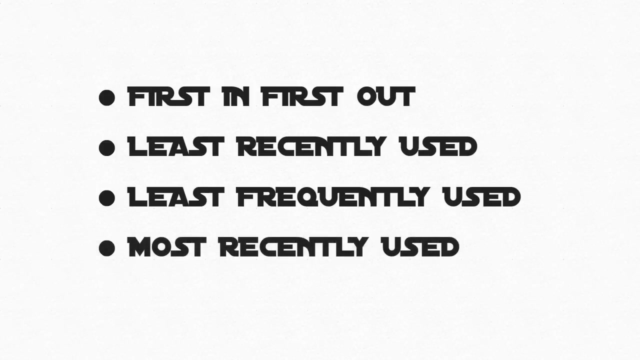 in memory, known as the status. The second to check if the page has been modified And a third to check if the page has been referenced recently. How do we determine replacement of pages? By using a page replacement policy. First in, first out, Least recently used, least frequently used and most recently used are replacement: 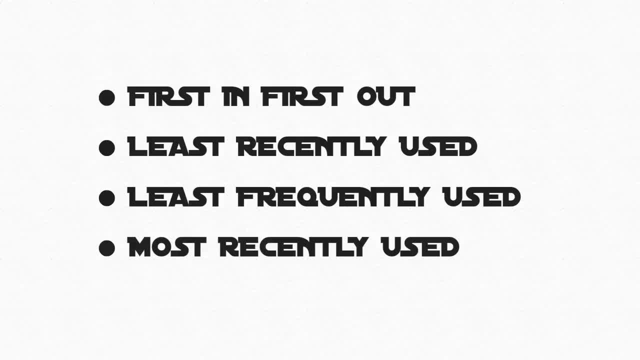 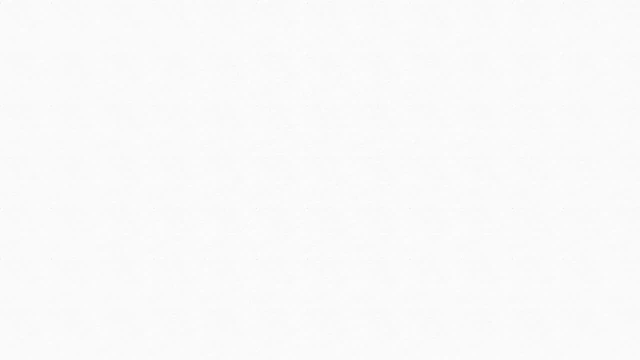 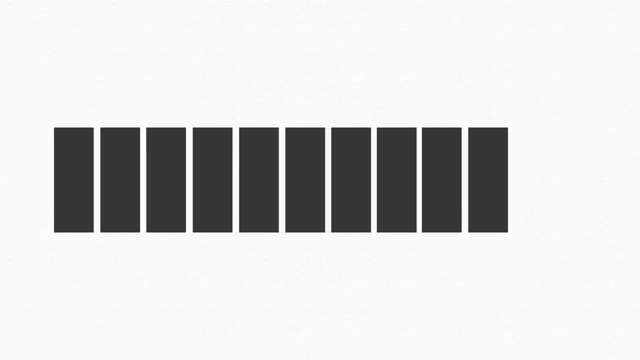 policies used to change pages based on a specific algorithm. These are all pretty self-explanatory and are crucial to the efficiency of the system. So we have looked at page map allocation and demand paging. But what else is there? Well, we have looked at separating the jobs into 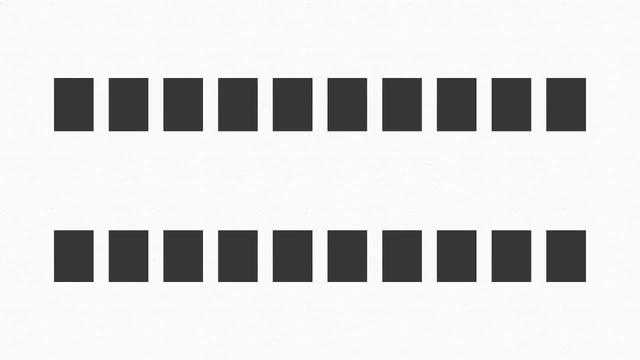 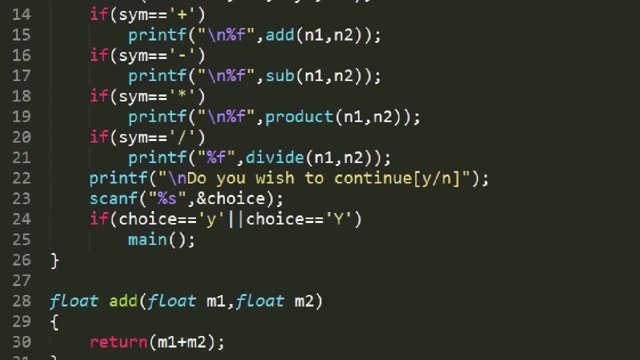 separate pages. What if we could break it down even further? We can. Segmented memory allocation splits the job into separate segments that reflect the nature and structure of the code. Usually, when you view a script, it is separated into individual functions or subroutines that can be called one at a time. You 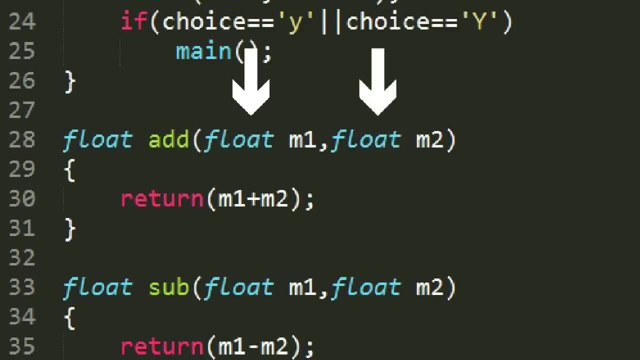 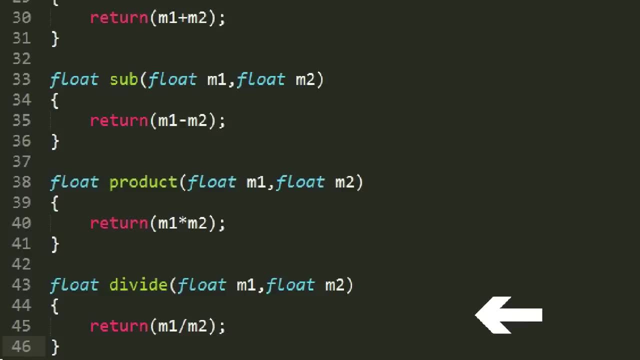 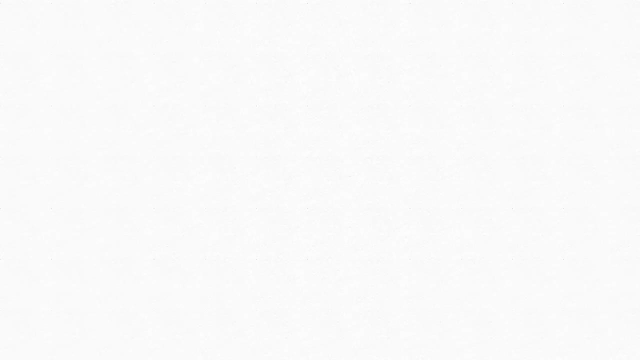 may have a function called ADD that makes a calculation of two numbers, And a function called DIVIDE. We can call these one after the other and they will run in the chosen order. Now take all of these functions and label them as segments. Instead of using a page map table, we now have a segment map table.